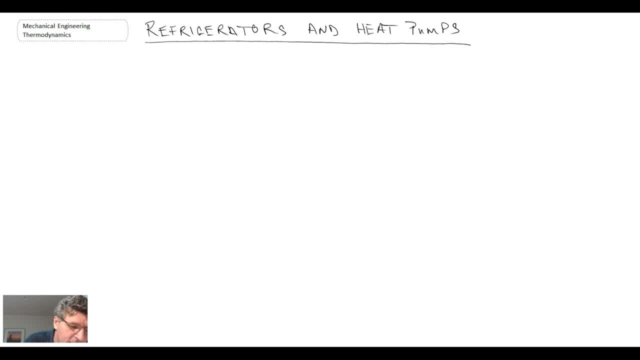 A refrigerator and heat pump are basically the exact opposite. So these are devices that take heat from a low-temperature source temperature and move it to a hotter temperature medium. so schematically, just like we did before, we looked at the heat engine, what we'll do now is we'll sketch. 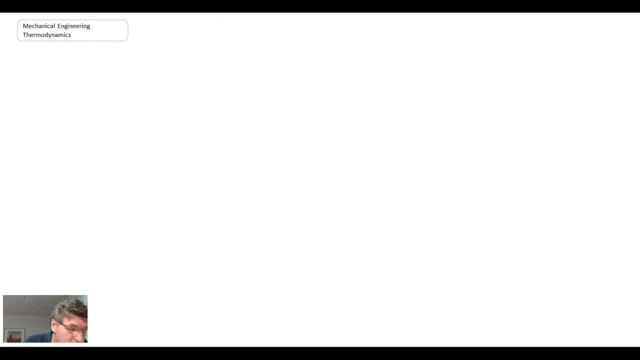 out the heat pump. so for a heat pump, I'll put it here in a circle and we're putting energy in or work in, so we have some network coming in. and then down at the bottom we have a sink which is at a low temperature and heat is flowing from. 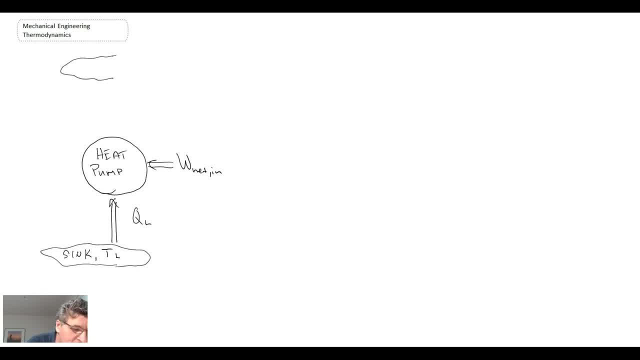 the sink and it's flowing up to a source which is a high temperature source, and then here we have heat going up to the source. so it's going in the opposite direction that we saw for the heat engine earlier. now, in terms of a schematic of a cycle, 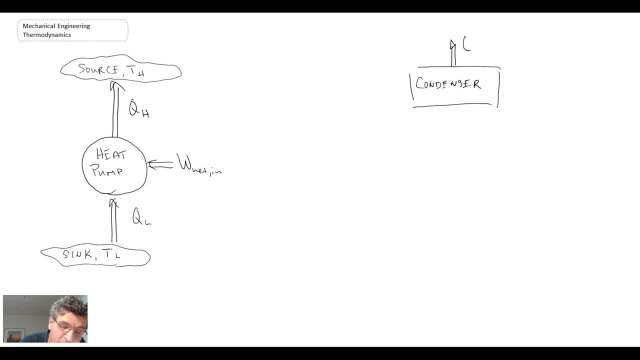 we would have a condenser whereby our working fluid is rejected heat before that in the process. what we would have is a compressor, so the fluid is coming out of the compressor and flowing into the condenser, and here is where we do our network in you state. 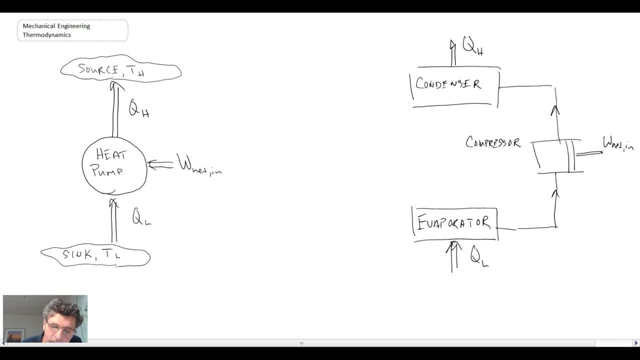 we have an elevator and that's where the low c temperature heat source is coming in, and then, after the condenser we come out and here we have an expansion valve for an oil handler. have an expansion valve or a throttling valve where we lower the pressure. so if 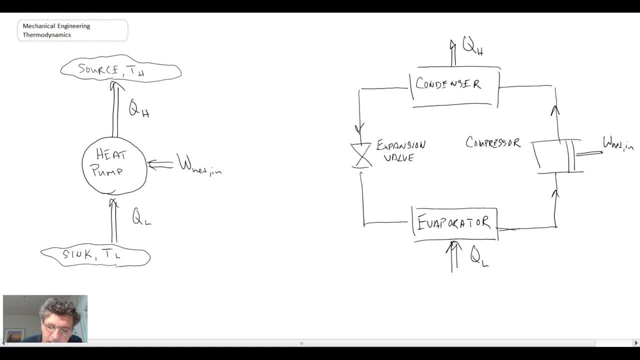 you recall the lecture where I was talking about the uniform flow process and I showed you a video of air coming out of a compressed tank. we saw water and we also saw ice. that's essentially what was going on. there was this type of cycle. we had a compressor. it goes into a tank. it's hotter than the environment. so 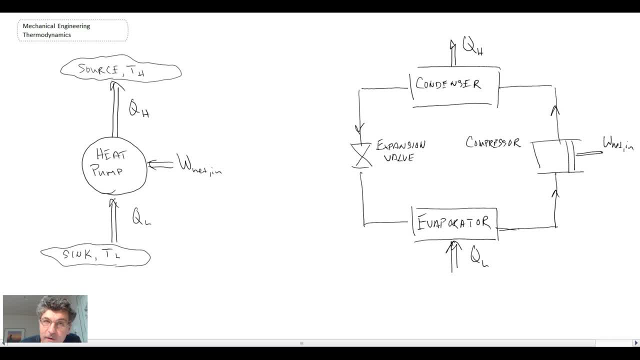 it rejects heat to the environment. I then open a valve. very quickly. it expands, it gets cold, and when it's cold, that's when you can absorb heat from the surrounding environment. so, depending on the particular application that you're looking at here, if the location where the heat was coming from, so you're 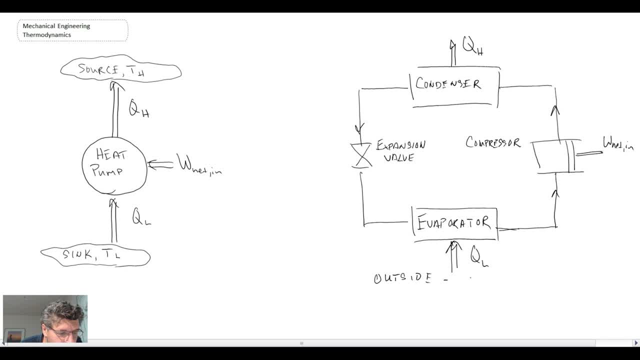 saying that the air is coming out of a compressed tank and you're looking at the outside. that would be an example of a heat pump. if you've ever stayed in a hotel or a motel where they have an air conditioning unit in the window, they can flip the switch from cool to heat. that's basically a heat pump there. they're less. 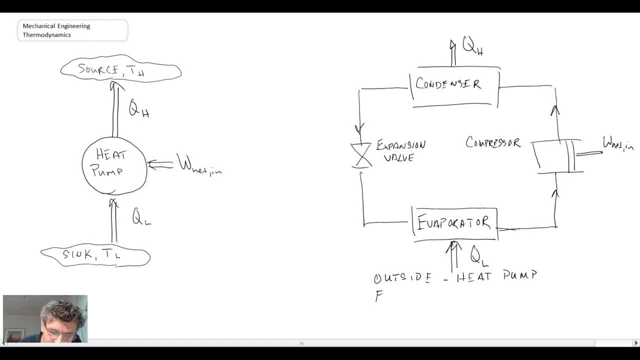 common in Canada than they are in the United States. and if it is food, then that would be a refrigerator. so that is the idea of a refrigeration cycle and a heat pump. now, in terms of the efficiency of this cycle, work net in is equal to QH minus QL. 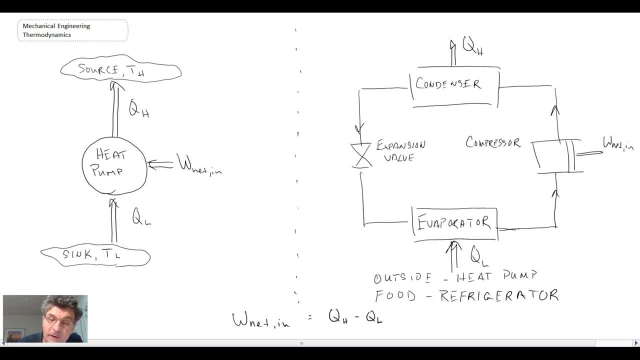 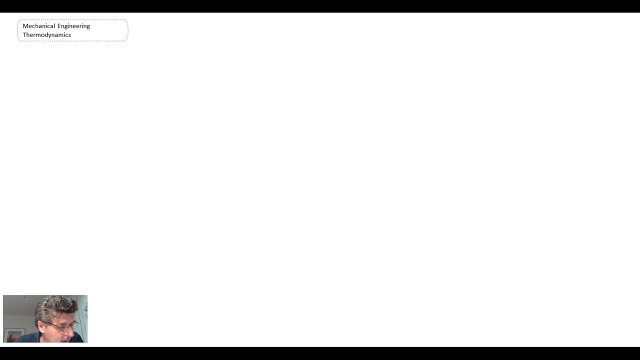 that is an expression that we will now use to determine or quantify how well the cycle is working. now for a heat engine. we talked about the efficiency, the thermal efficiency, of the cycle. for a heat pump or refrigerator, what we'll be talking about is the coefficient of performance. 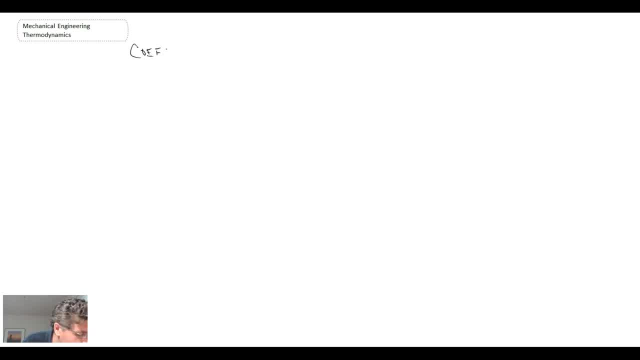 and this is written out in terms of a capital, COP, and what it is is our desired output divided by the required input. so, looking at a refrigerator, we would have the coefficient of performance of a refrigerator. ill write it as COP. subscript capital R, QL is the design. 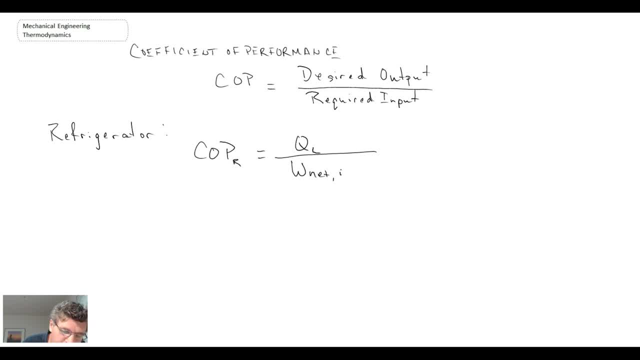 required and the required input is the work that we have to do, which we could then rewrite that as, So that becomes an expression for the coefficient of performance of a refrigerator and similarly for a heat pump. So we can substitute for the network N using QH minus QL and rearranging that, what we 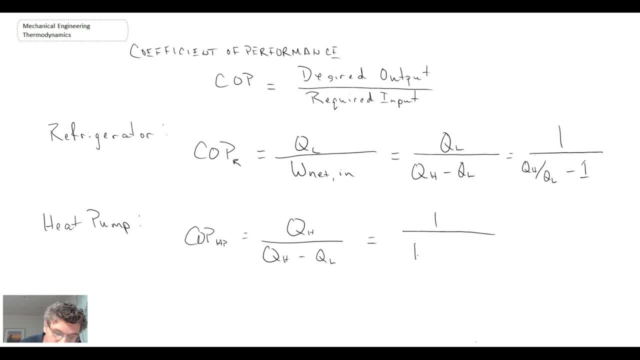 obtain is this expression. So you see, it's a little different depending if you're dealing with either a refrigerator or a heat pump. Typically, values that you'll find for coefficient of performance of heat pumps, they're going to be on the range of 2 to 3, and it would depend upon the working fluid and the design. 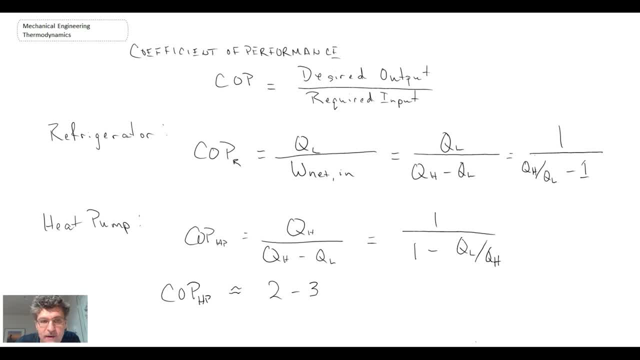 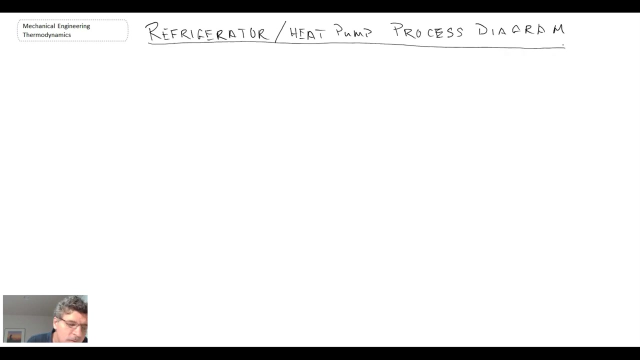 of the system. Just like heat engines have different efficiencies, You'll find a variety of different efficiencies or coefficients of performance for heat engines. So looking at this in terms of a process diagram, So sketching it out again, We had our condenser. 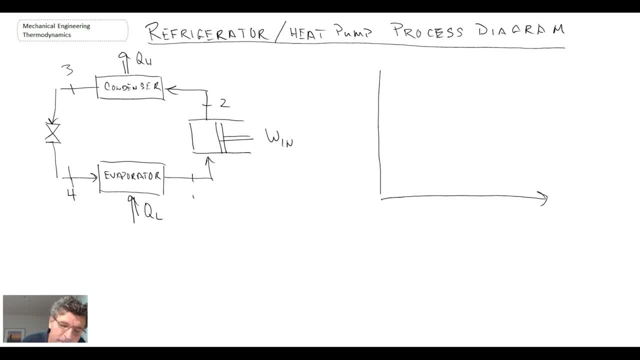 Now writing it in terms of a TS diagram. What I'll do is map it. I'll give it a name. It's a little bit more complex: map the state information to a TS diagram or, sorry, TV. so with this process we start over here at one. typically we go into a compressor. 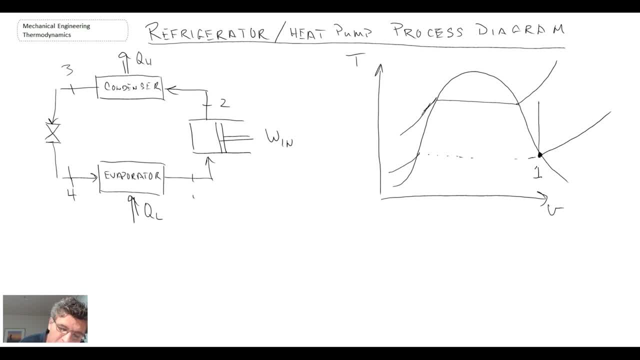 and so in the compression process we increase in temperature and that takes us up to state two. once we're in state two, and in here we're doing work, so we have work coming in. once we're at state two, usually we're at a hotter temperature than our surrounding environment. 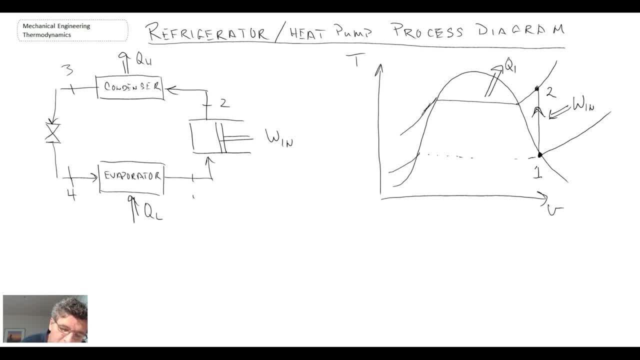 and so we reject heat to the surrounding environment, or we heat in the case of a heat pump. so we're moving in this direction now, and let's assume that we end at the compressed liquid line, so that would be at point three- we then go into a throttling valve, and a throttling valve is actually a constant. 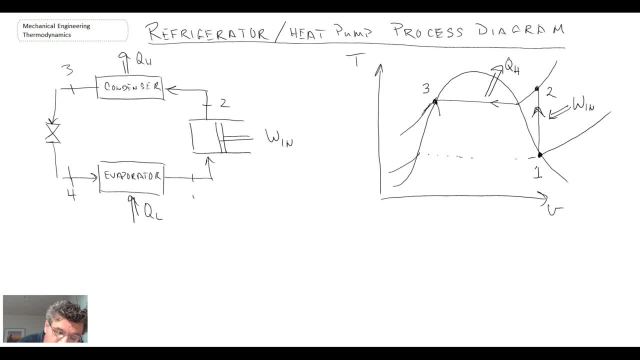 constant enthalpy process, but it will bring us down, something like that, to state three, and then we're going to go into the compression process and that's going to be at point four, and now we are at a lower temperature and consequently what we're able to do is absorb heat through this process here. so